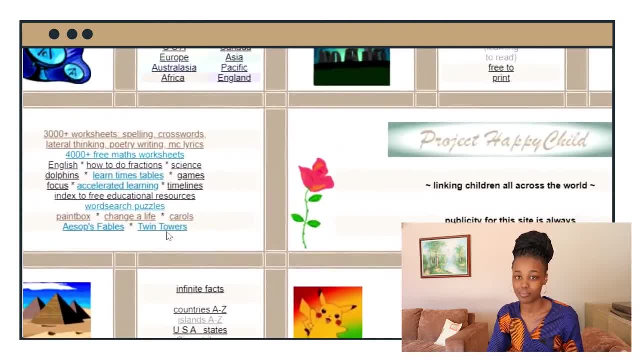 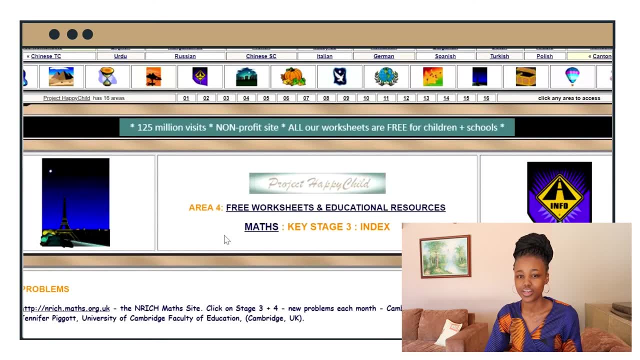 There are a ton of worksheets and post papers and exam papers that your child can look into on that website. One thing you should take note of, though, is that the user interface is not that great. It's quite confusing, especially if your child is young. 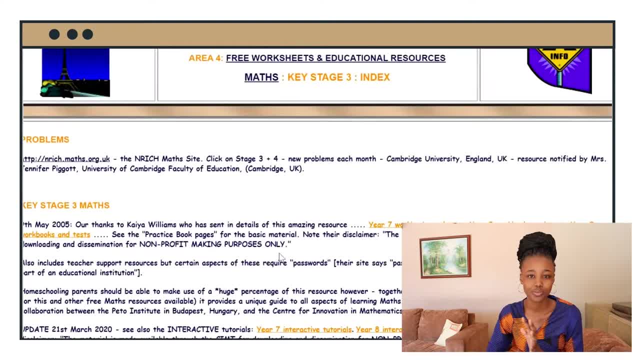 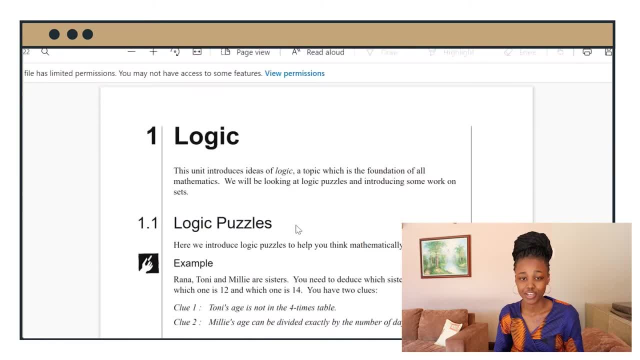 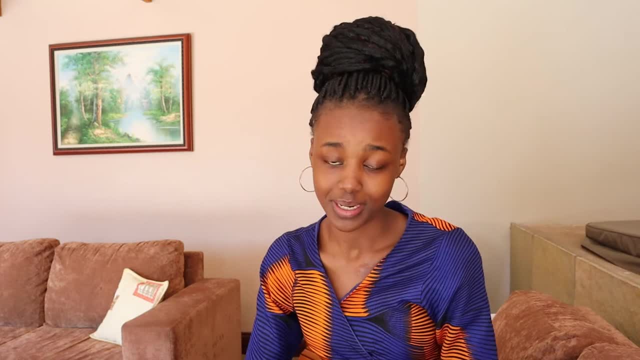 They might struggle with it a bit, being able to navigate through the website. as you can see it's it's quite. yeah, it's not very neat, but other than that, as you get used to it, it's quite easy to navigate through and it is a website that i highly recommend. website number two on my list of favorite. 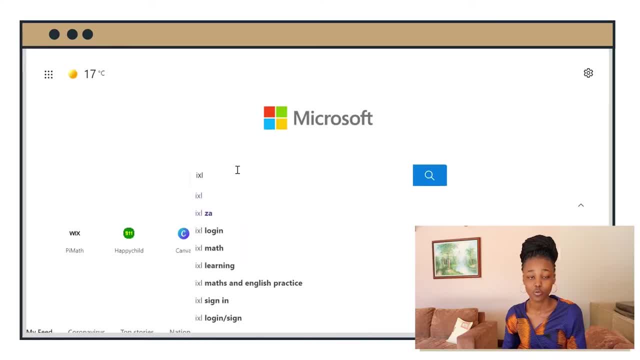 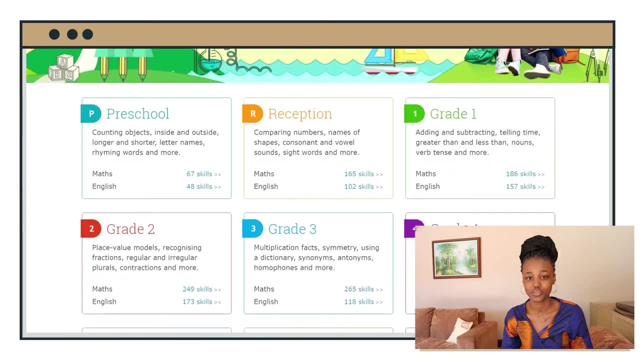 websites is i excel. this resource is awesome for practicing mathematics, and this one is great because it is clear and neat, very easy to navigate through, so it's something that your young child can also navigate through on their own. everything is laid out very nicely, especially the practice. 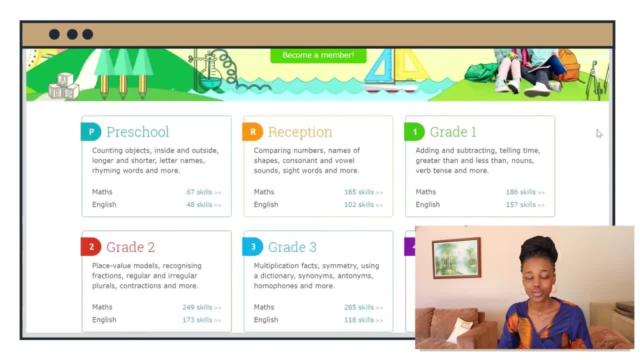 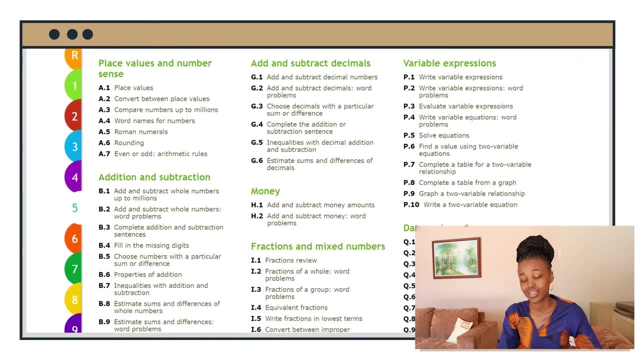 questions. they are categorized by grade levels, so it's super easy to find out which questions would be appropriate for your child. another thing i love about this website is that it's interactive. your child can log answers into i excel and it will tell them whether the answer they gave was. 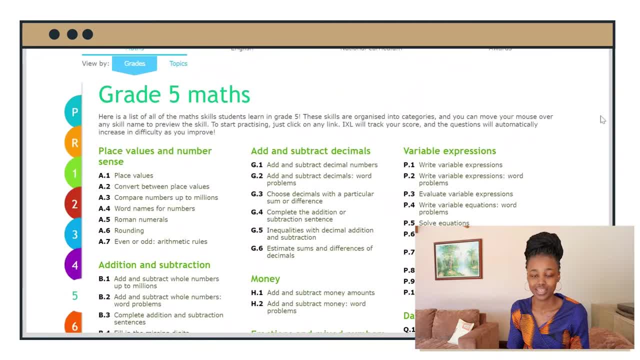 wrong or right. if it was incorrect, your child will then get feedback as to why the answer was wrong. this, by the way, is the free version. they do have a paid version, but the free version has worked out very well for me, so i don't know what additional features you can find on the. 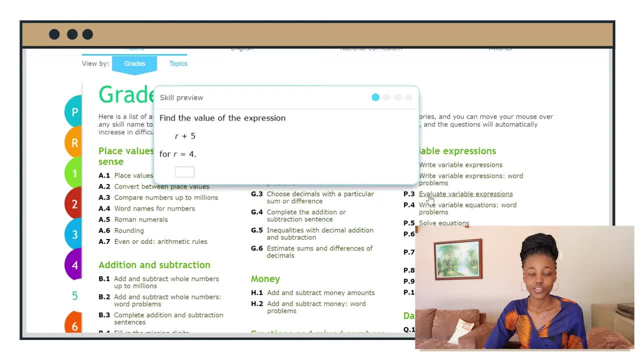 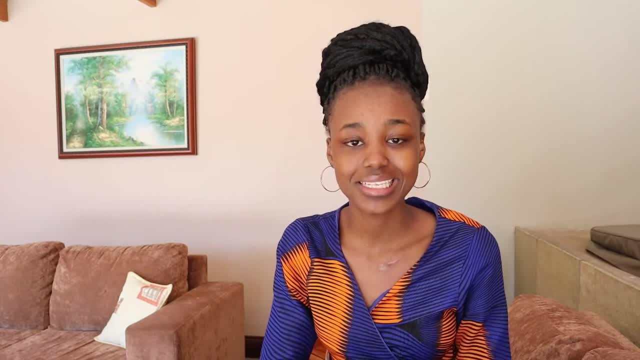 paid version, but i'm sure they do enhance your experience. it's an awesome resource for young kids and you can go ahead and check it out now. my number one favorite math website is mathisfuncom. this website is brilliant. the reason i love this website so much is that it doesn't just 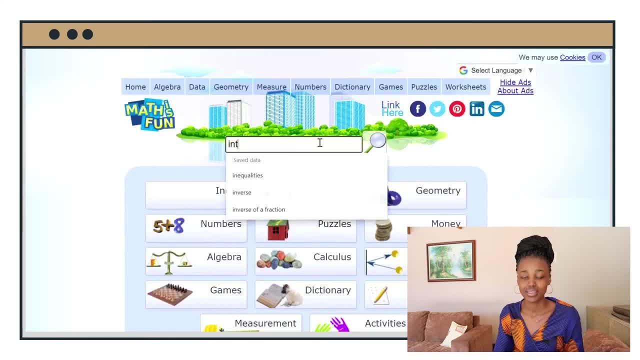 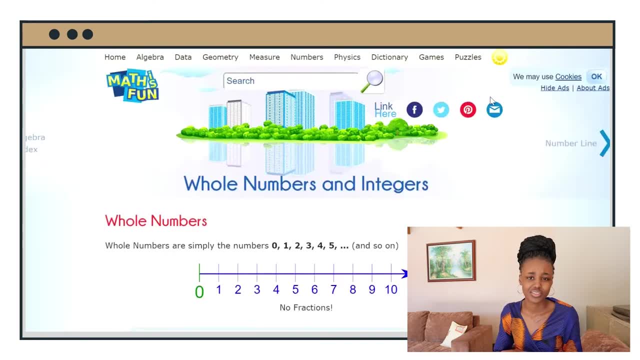 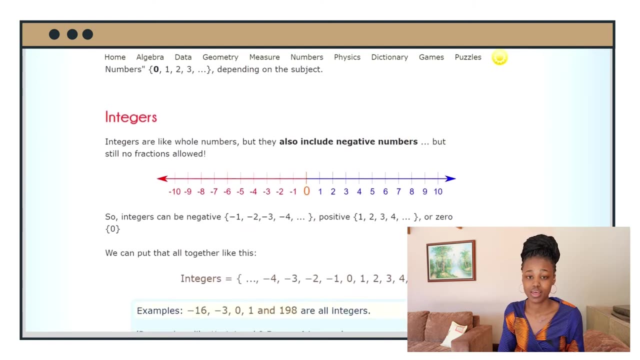 teach children math, but it helps them to understand it by teaching the math principles, which is exactly what young kids need to gain a point in their life. they use pictures and illustrations, all with the aim of helping your child understand math concepts. your child can also practice math on this website, because they do have practice questions on there. 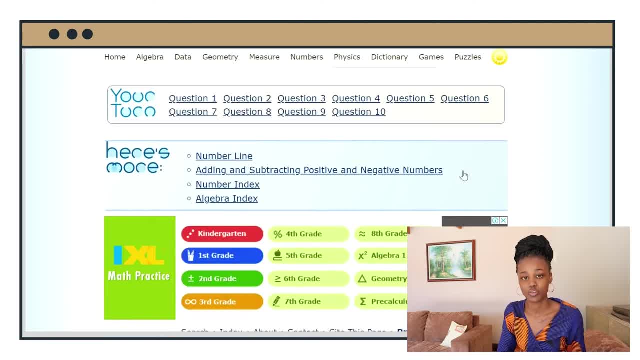 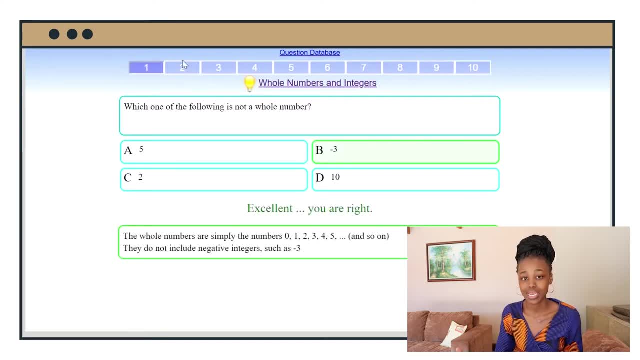 at the end of each lesson. although i do not necessarily use that feature of the website, they do have quite a few good practice questions on there. overall, it's an incredible website and it's my number one free math website- parents, if you know of any good math websites or math resources.